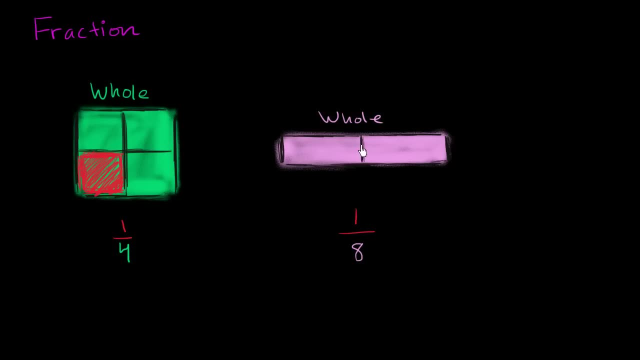 So here I've divided into two equal parts. That looks pretty good, And now I can divide each of those into two equal parts to get me four equal parts. And then, if I were to divide each of those into two equal parts, I will have eight equal parts. 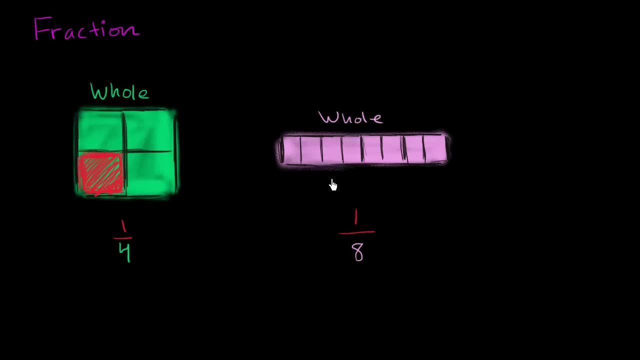 And it's not exact. Obviously I've drawn it by hand, But hopefully this gets you the sense. So now I have eight equal parts, Eight equal parts, And now I'm going to select exactly one of them, And that'll represent 1 eighth. 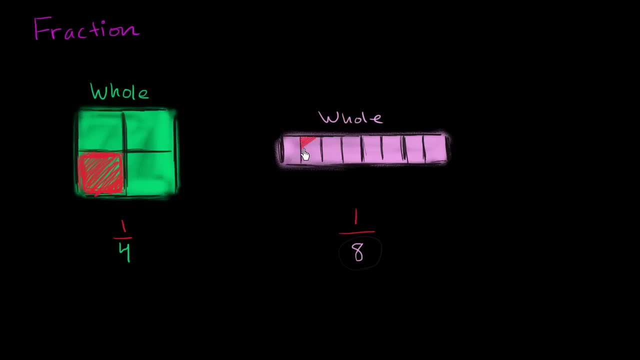 And I could select any one of these, But I'll just do this one to show you. it does not have to be necessarily the first one. So, once again, this square right over here that I'm shading in red represents 1 eighth. 1 eighth of the whole. 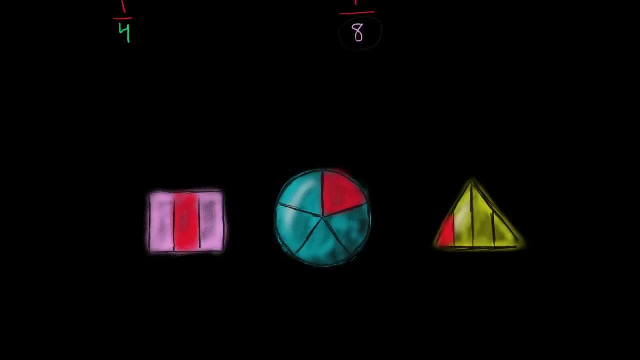 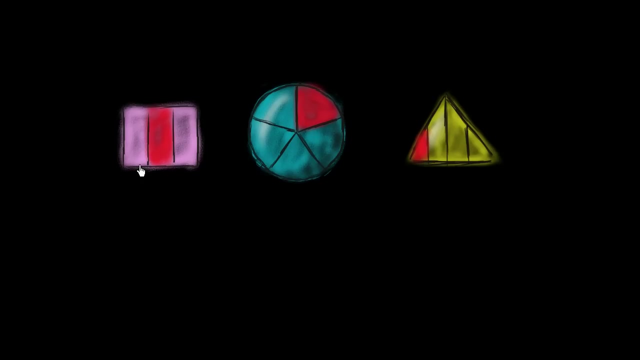 Now let's look at a few more examples where I've shaded them in ahead of time, And what I want you to do right now is pause the video And, either in your head or on a piece of paper, write down if you consider this purple thing, the whole. 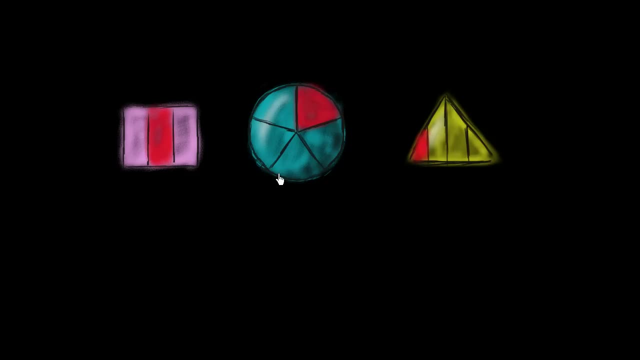 what fraction does this red part represent? If you consider this blue part the whole, what fraction does this red part represent? If you view this yellow triangle as a whole, what fraction does this red part represent? And so I encourage you to pause the video. 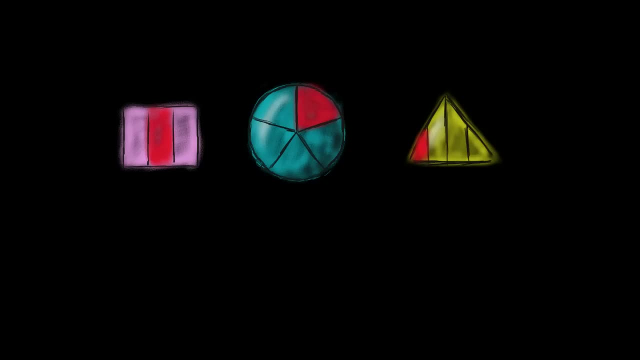 Now let's look at each of these. So in this case, for this rectangle, we have three equal parts And we've shaded in one of them. So this red rectangle right over here represents 1 third of the whole. Now, over here, in this kind of pie-looking thing, 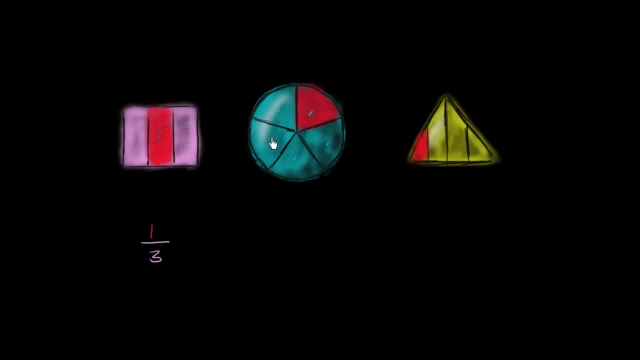 this circle-looking thing. we have 1,, 2,, 3,, 4,, 5 equal parts Shaded in one of those five equal parts. So this little slice of the pie, this represents 1 fifth. This right over here is 1 fifth of the entire pie. 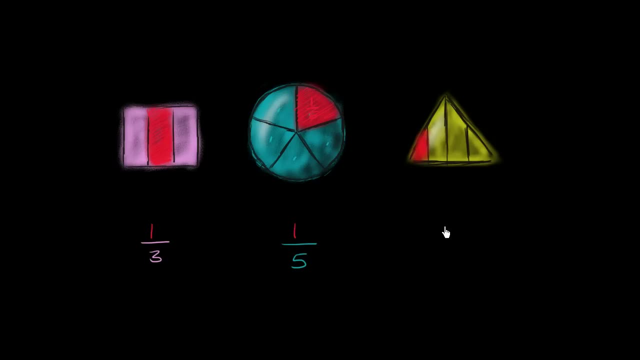 Now this one's interesting. You might be tempted to say, well, I've got four parts And then I've shaded in one. That must represent 1 fourth. But remember it needs to be four equal parts And it's pretty clear. looking at this.